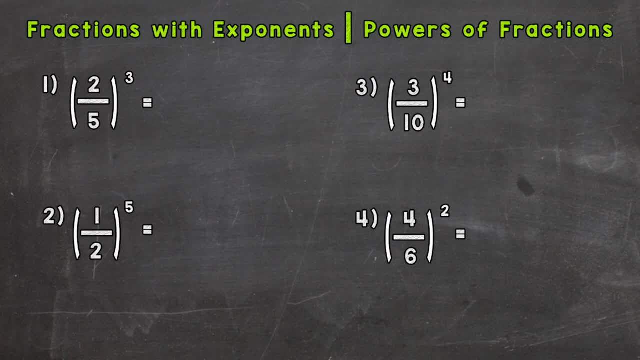 where we have two-fifths to the power of three. Now, two-fifths is our base and we need to expand it out- the number of times that the exponent indicates, And our exponent is three. So that means we need to multiply two-fifths by itself three times. So it looks like this: Two-fifths. 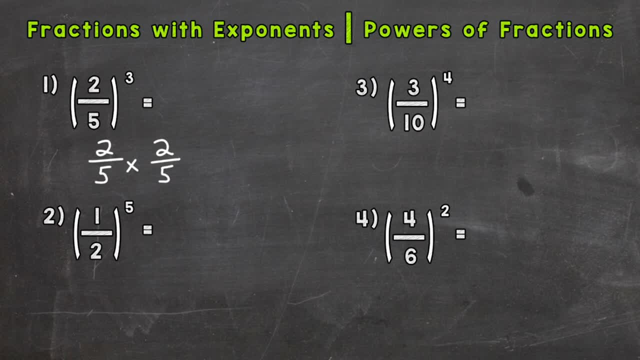 times, two-fifths times two-fifths. This problem that that exponent of three does not mean two-fifths times three, It means expand the base, or two-fifths out, three times. Now we're ready to solve. So it's just multiplying. 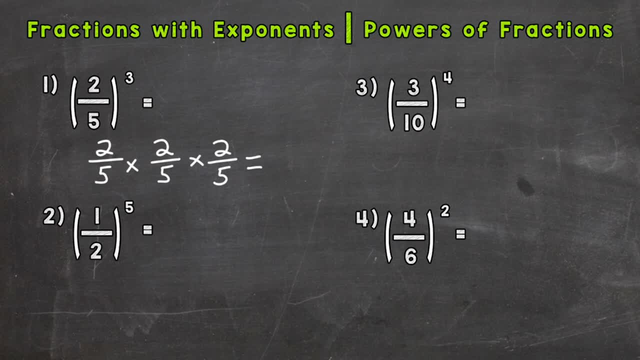 fractions at this point, which is multiply straight across. So 2 times 2 is 4 times 2 is 8.. 5 times 5 is 25, times 5 is 125.. So our answer is 8 over 125.. 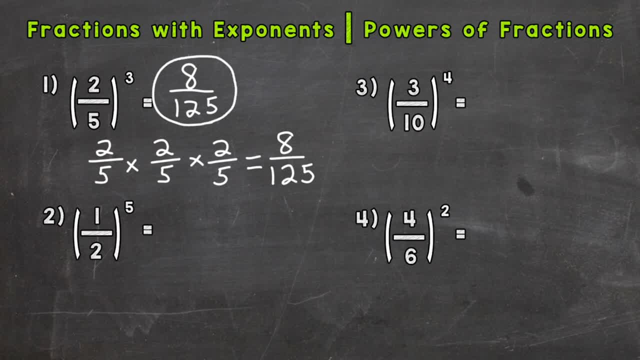 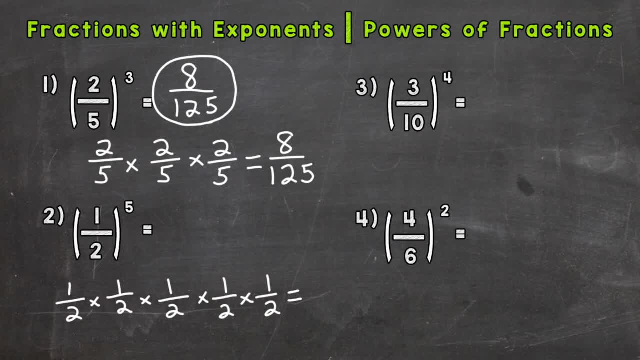 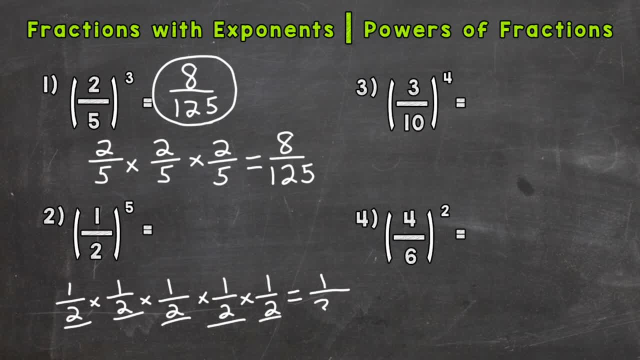 Times two is 32.. So we get one over 32 for our one half to the fifth power, Number three, three tenths to the power of four or to the fourth power. So let's expand three tenths out four times and solve. 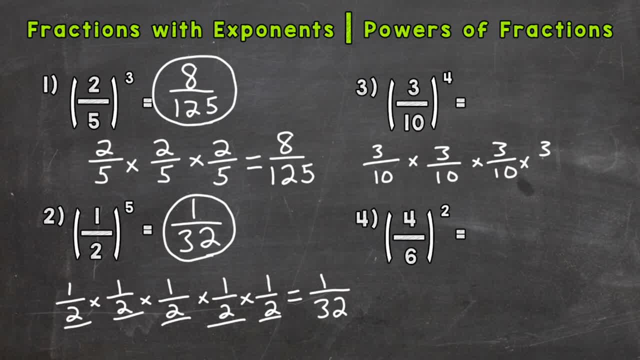 All right, we are ready to go here with three. times three is nine. Times three is 27.. Times three is 81.. Now for the denominators of ten. Ten times ten is a hundred. Times ten is a thousand. Times ten is ten thousand. 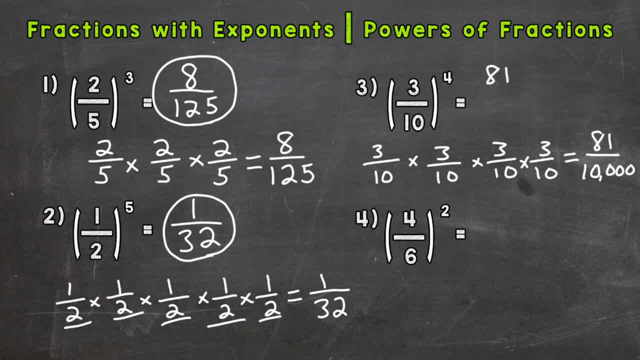 So we get 80.. So we get 81 over 10,000.. And lastly, number four, four over six to the power of two. So we expand four sixths out twice and multiply straight across. Four times four is 16.. 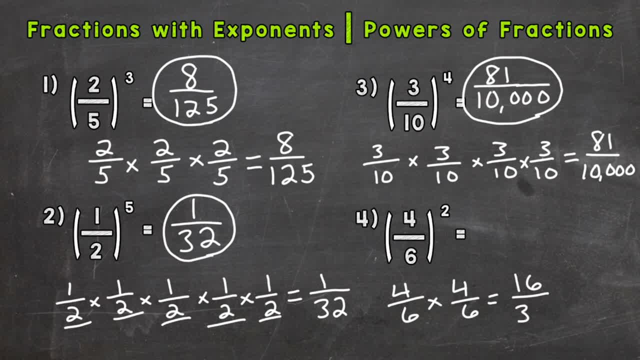 Six times six Is 36.. So 16, thirty-sixths, which can be simplified. We can divide both of those by two and get eight, eighteenths, which can be divided by two again, which gives us four, ninths, as our simplified version of 16 thirty-sixths. 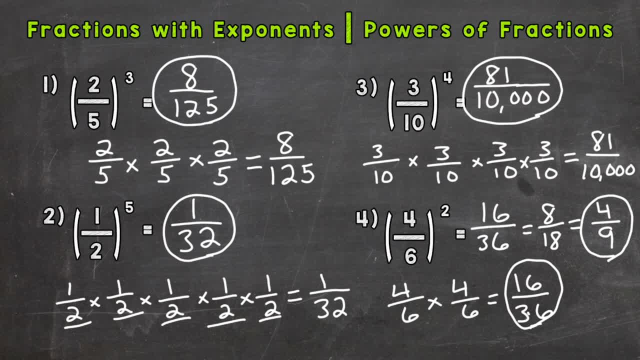 Or you could have divided 16 and 36, both by four right off the bat, and simplified in one step. So four ninths for number four, or the unsimplified answer of 16 thirty-sixths. So there you have it. 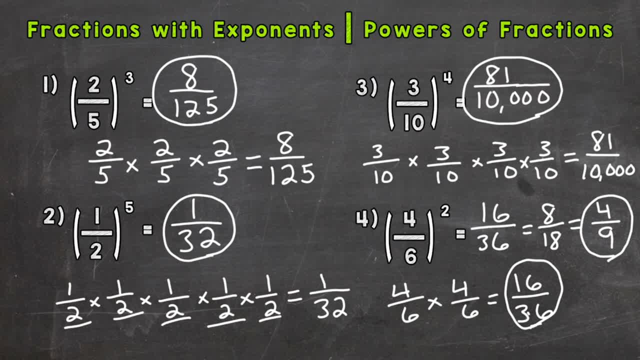 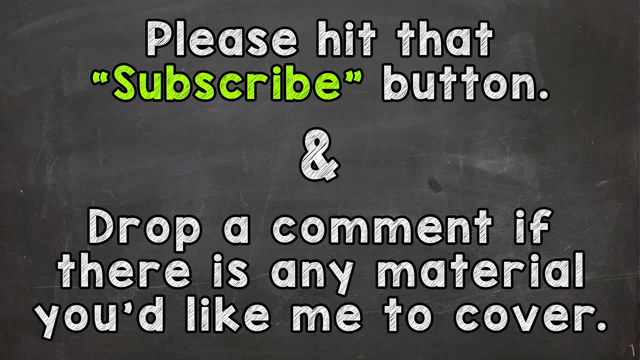 There's how you solve fractions with exponent problems. Hopefully that helped. Thanks so much for watching. Until next time, Peace, Bye, Bye, Bye, Bye, Bye, Bye, Bye.